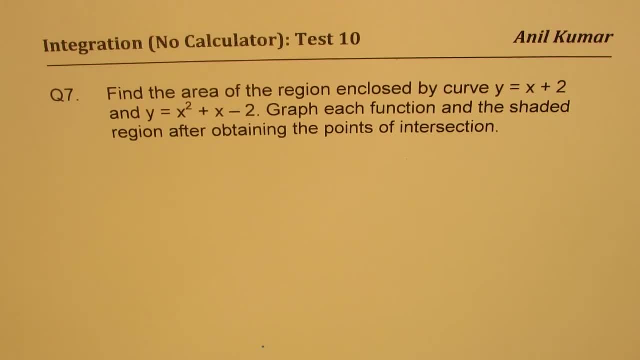 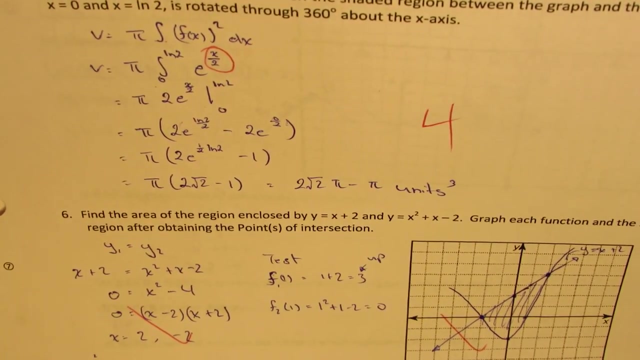 I am Anil Kumar. Welcome to my series on integration. To understand the concepts, we have taken up questions from previous test papers. Here is another excellent question from IB test paper. So we'll do question number 6 in this test paper, which is going to be question number 7 for us. 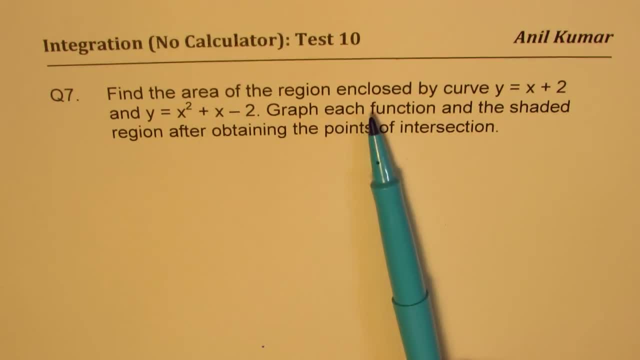 Question number 7.. Find the area of the region enclosed by curve. y equals to x plus 2 and y equals to x square plus x minus 2.. Graph each function and the shaded region. after obtaining the points of intersection, You can always pause the video and answer the question. 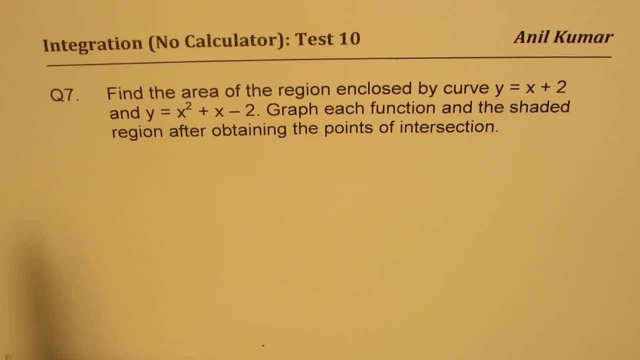 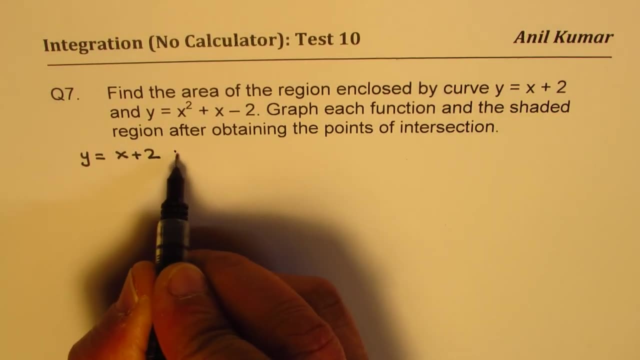 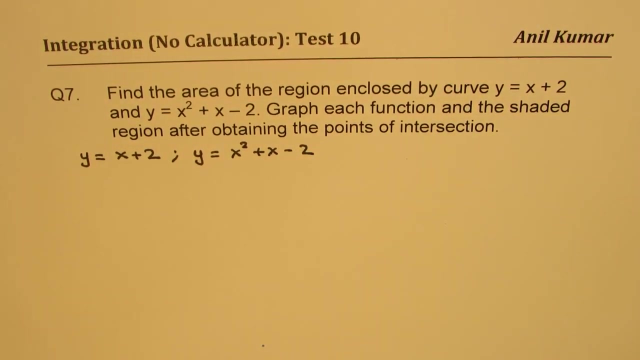 So let's first find the point of intersection between these two curves. So we are given y equals to x plus 2.. And we are also given that y is equal to x square plus x minus 2.. So at the point of intersection these two values should be seen. 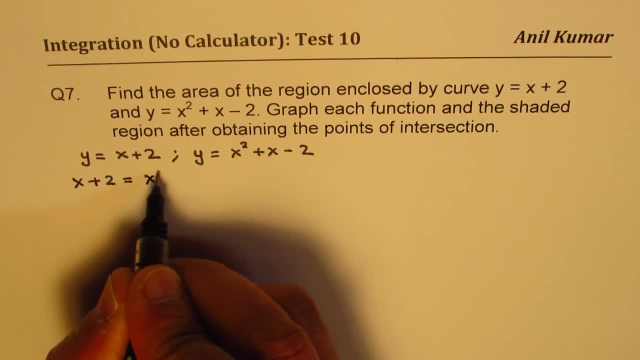 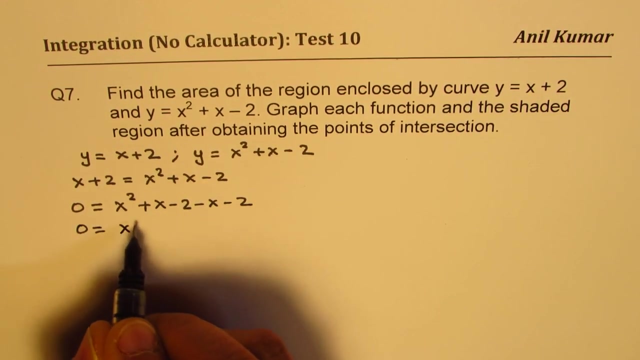 So we'll write: x plus 2 equals to x square plus x minus 2.. Bringing them together, we can write 0 equals to x square plus x minus 2 minus x minus 2. And that gives us x square plus x minus x cancels and we get minus 4.. 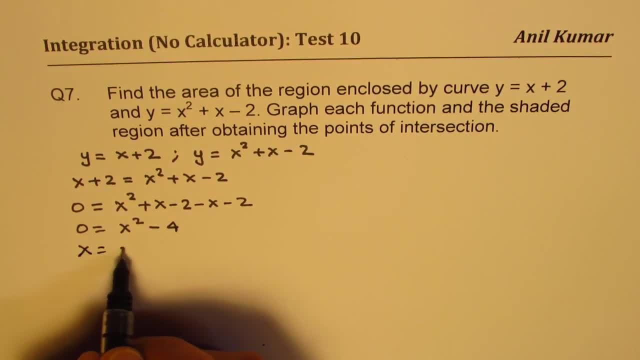 So that gives us two values of x. So x is equal to plus minus 2, right square root of 4.. So these are the two points of intersections. Now we will sketch both the graphs. Let me make a small sketch here. 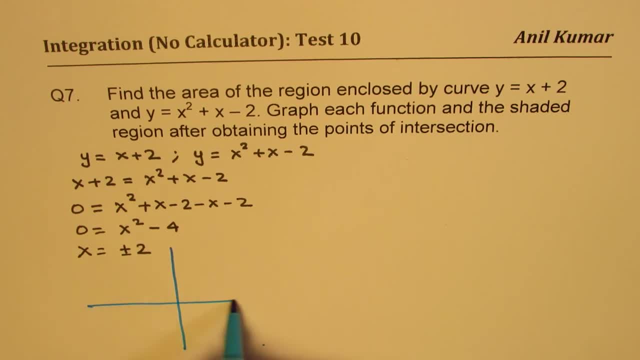 Then we'll find the area on the right side. So one of the curves is a straight line. y equals to x plus 2, right. So let's say this is 1, this is 2.. So we'll just draw a straight line here. 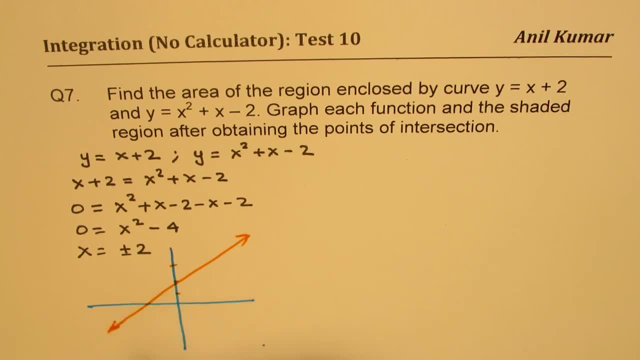 So our drawings will be slightly approximate, right, But I hope they'll give you a fairly good idea about what we're trying to do. So this point here is: the intercept is at minus 2.. Here the y is equal to x. The y-intercept is at plus 2.. 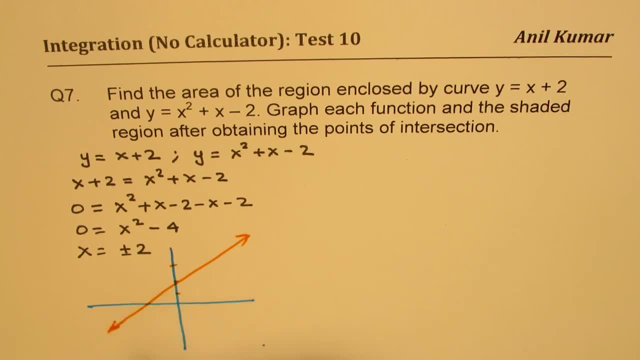 So our drawings will be slightly approximate, right, But I hope they'll give you a fairly good idea about what we're trying to do. So this point here is: the intercept is at minus 2.. Here the y is equal to x. The y-intercept is at plus 2.. 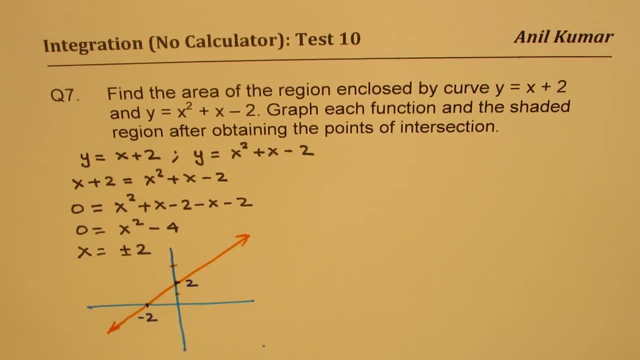 The points of intersection between the parabola and the line are at plus minus 2.. That means one of this point is here, The other one will be on this side, right? So let's say this is 1.. So at 2, somewhere here, right? 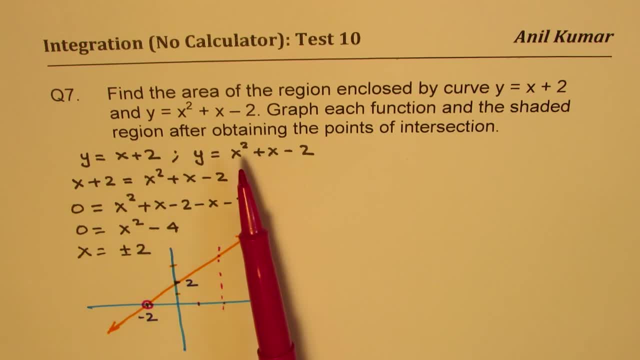 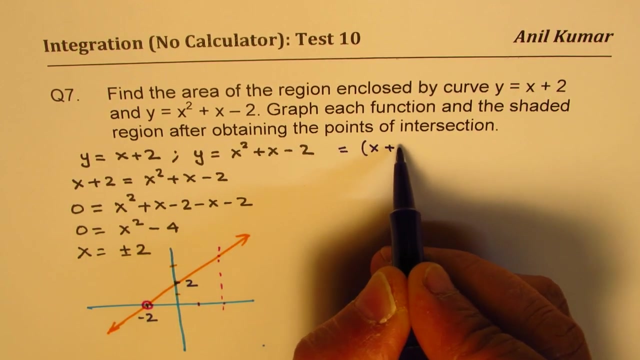 Somewhere here. Okay, Now let's look into the second equation, which is x square plus x minus 2.. The equation is x square plus x minus 2.. So the equation x square minus x minus 2 can be factored and we can write this as x plus 2 times x minus 1, right. 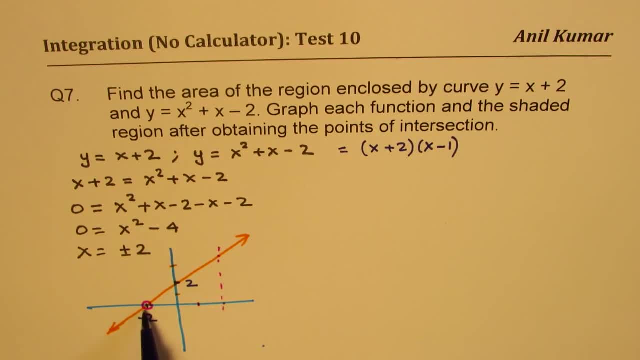 So that means we have a 0 at minus 2, as expected, and the other one is at 1, right, So we have two 0s for this parabola. So the vertex will be somewhere along this line. So let me just sketch a parabola here going through these points. 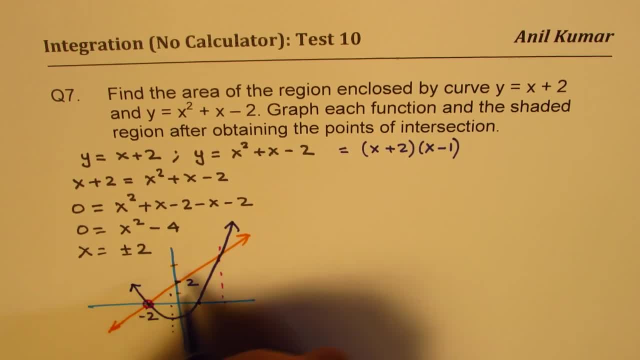 And then through the intersection. It doesn't make sense to you, right? So this point is the point of intersection. where x equals to 2, correct Area between the curves will be this shaded portion clear. So we won't define area of this curve. 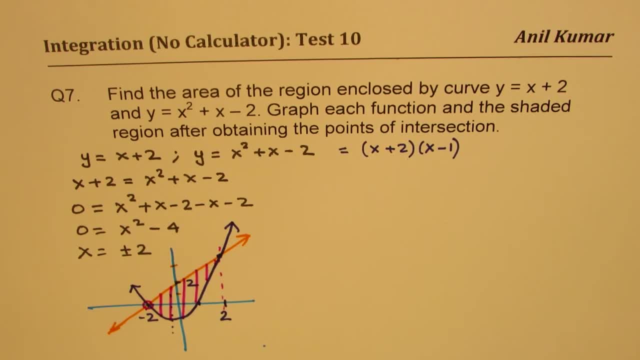 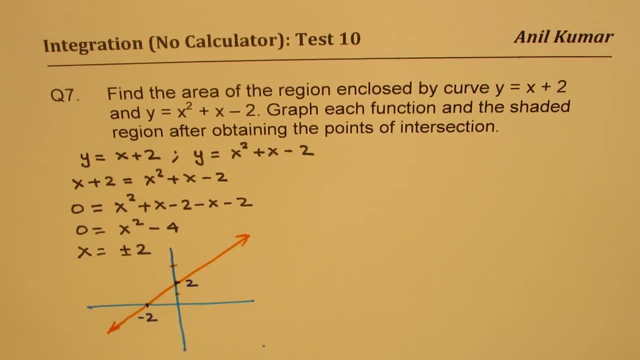 The points of intersection between the parabola and the line are at plus minus 2.. That means one of this point is here, The other one will be on this side, right? So let's say this is 1.. So at 2, somewhere here, right? 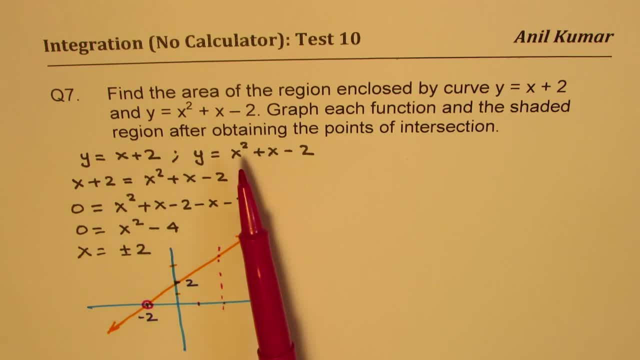 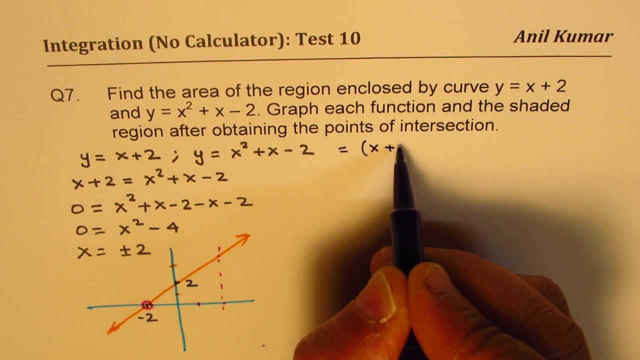 Somewhere here. Okay, Now let's look into the second equation, which is x square plus x minus 2.. The equation x square minus x minus 2 can be factored and we can write this as x plus 2 times x minus 1, right. 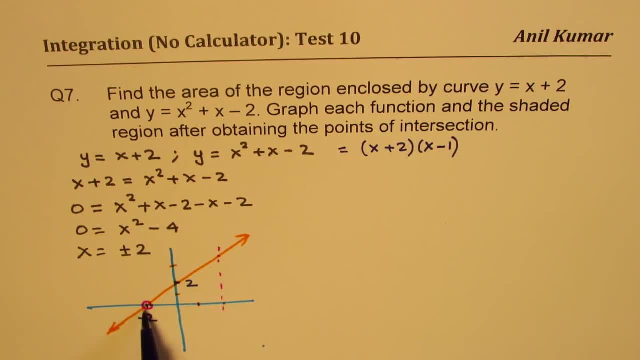 So that means we have a 0 at minus 2, as expected, and the other one is at 1, right, So we have two 0s for this parabola. So the vertex will be somewhere along this line. So let me just sketch a parabola. 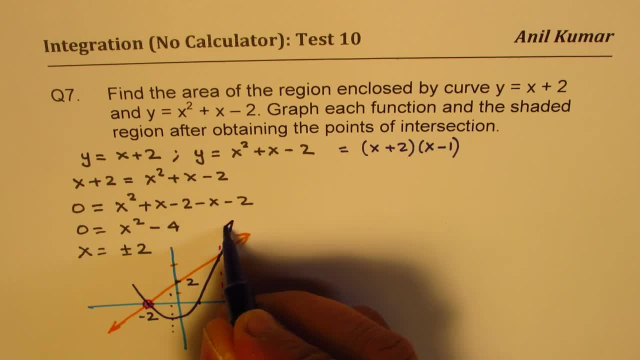 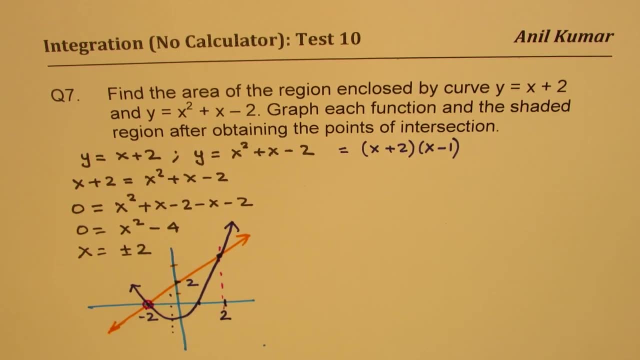 Here. going through these points and then through the intersection Doesn't make sense to you, right? So this point is the point of intersection. where x equals to 2, correct Area between the curves will be this shaded portion clear. 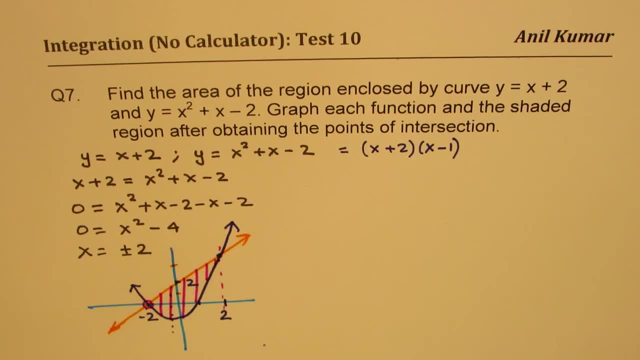 So we won't define area of this curve. So definitely the area of this curve is- you can write this function minus the other function, right So to find the area, we can say that area of the curve will be equal to. 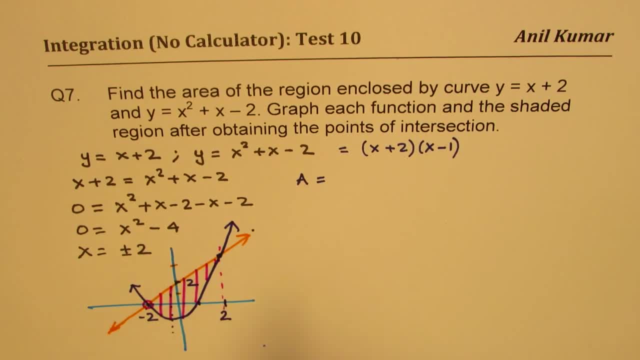 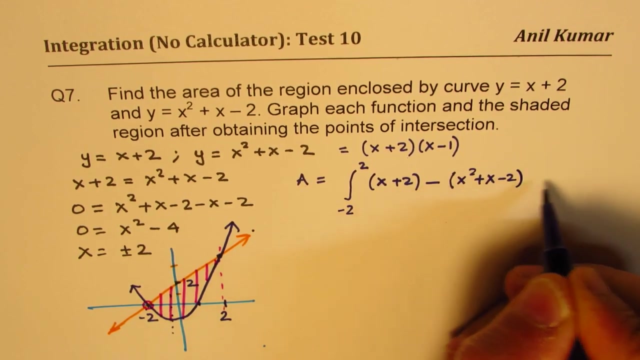 area between these two x values, that is integral, from minus 2 to 2.. And the function is going to be the linear function, which is x plus 2, take away the parabola right. And the function is going to be the linear function, which is x squared plus x minus 2, dx, correct. 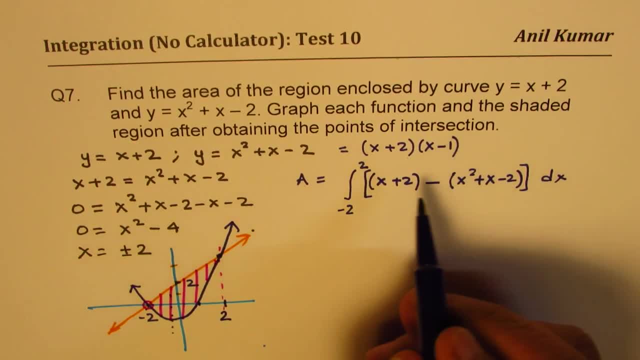 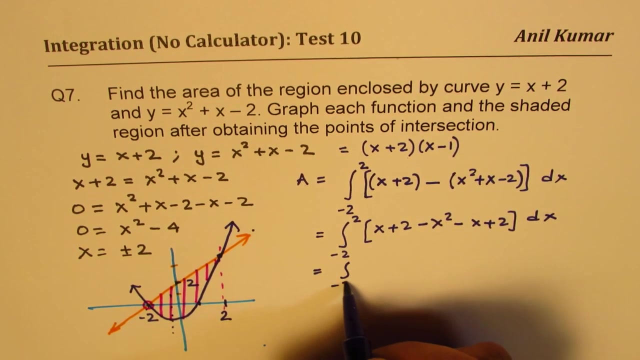 So that becomes the area under the curve. Let's try to simplify this. So what we get here is integral from minus 2 to 2, we have x plus 2 minus x, squared minus x plus 2, right dx. That is integral from minus 2 to 2.. 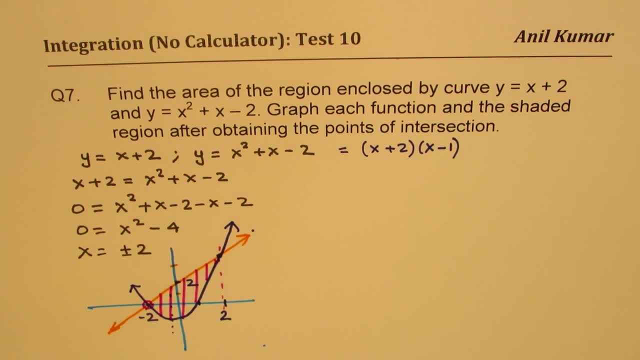 So to find the area, we can say that area of the curve will be equal to area between these two x values, that is integral from minus 2 to 2.. And the function is going to be the linear function, which is x plus 2.. 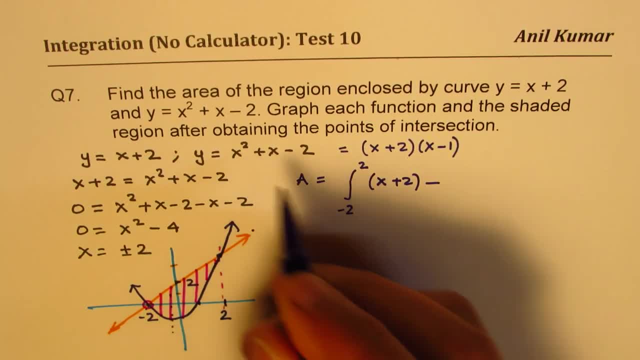 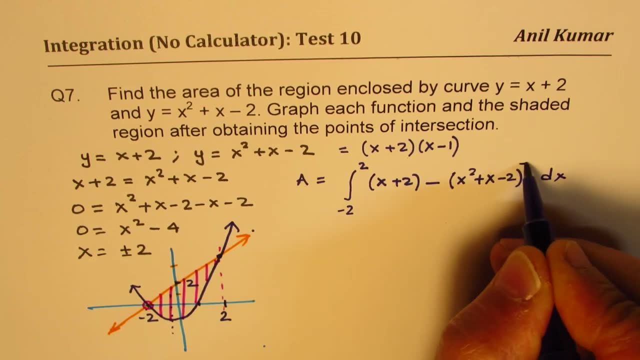 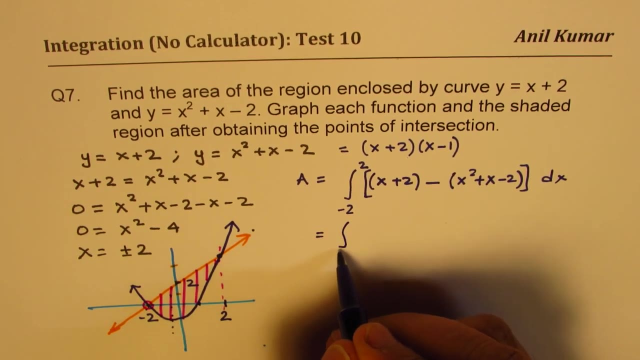 Take away the parabola right. So region between these two, Which is x squared plus x minus 2, dx, correct. So that becomes the area under the curve. Let's try to simplify this. So what we get here is integral from minus 2 to 2.. 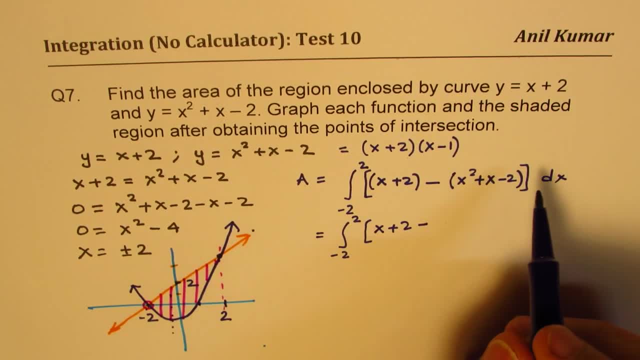 We have x plus 2 minus x squared, minus x plus 2, right dx, That is integral from minus 2 to 2.. And this gives us x and x cancel. We get minus x squared and 2 plus 2 is 4.. 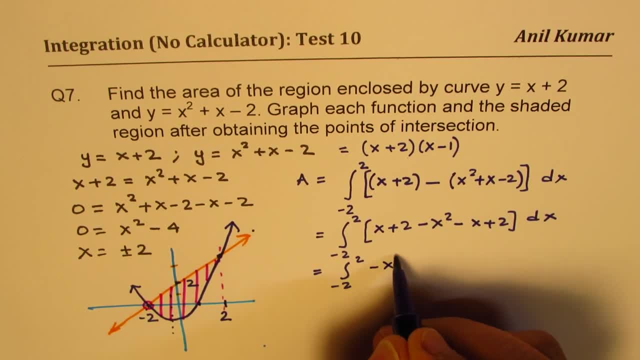 So we get minus x squared plus 4, right. The integral of this will be x cubed. Let's write down here: So we have minus of x cubed over 3.. 3 plus 4x, from minus 2 to 2, right. 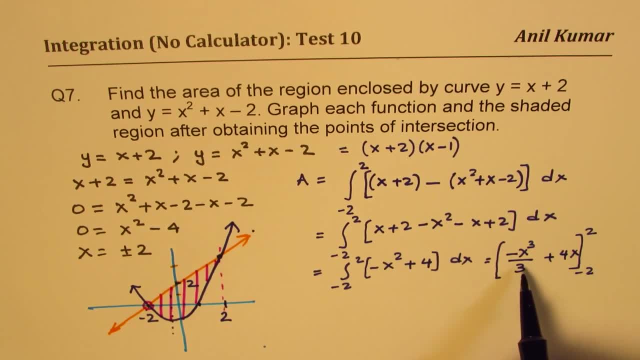 Substitute these values. So when you substitute these values, we get this as equal to minus of 2 cubed. Okay, so minus of 2 cubed, the denominator. let's write down here: minus, So minus, and minus becomes plus right. 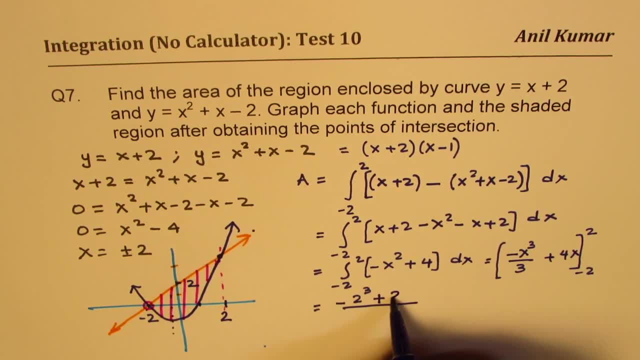 Because the cube will be negative of 2 cubed over 3.. And for this we get plus 4 times 2. minus of minus 2 will be plus 2, right, So that becomes the integral for us. So this minus we'll take outside actually. 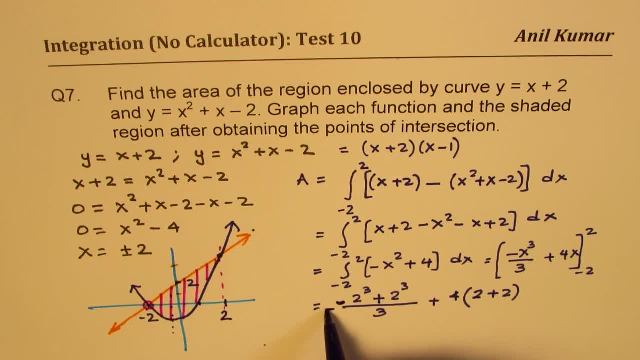 2 cubed will give us x squared 2 cubed will give us a negative value. Let me write minus like this, right? So so which is equal to 8 and 8, 16.. So we get minus 16 over 3, and that is 2 and 2, 4, 4 times 4 has 16, right. 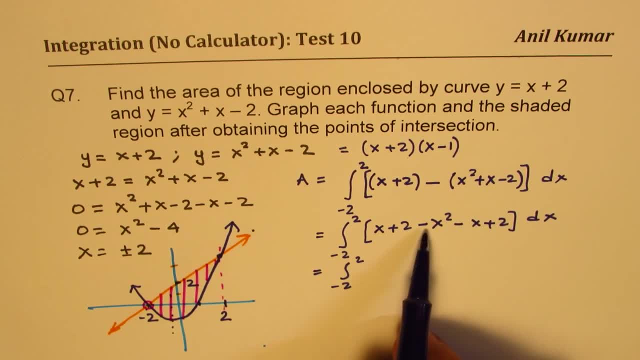 And this gives us x and x cancel. we get minus x squared and 2 plus 2 is 4.. So we get minus x squared plus 4, right? The integral of this will be x cubed. let's write down here: 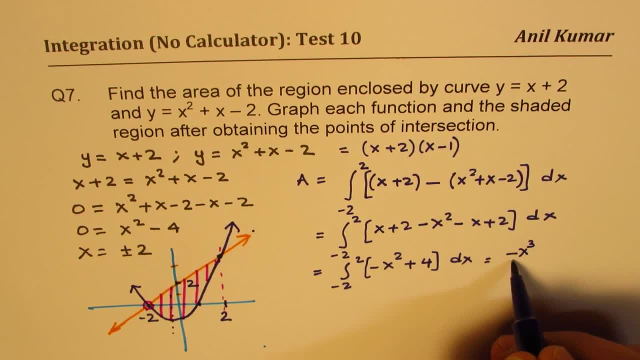 So we have minus of x cubed over 3.. So that's the integral minus cos representa x squared right. So this is the contradiction of the of the integral sin squared over 3. Our radians, that's something that. So we're essentially going to be positive 1 over 2.. All right Now. why don't we ropes? eram Пр트가. Why don't we Jaquest? Yeah, Why don't we Jaquest? Why don't we Jaquest? Why don't we Jaquest? Well, you're right, Bar sailing that. 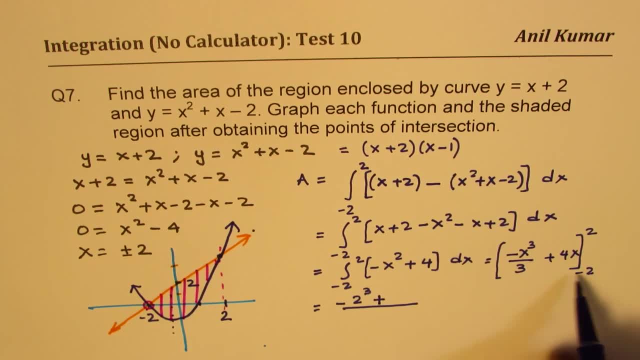 Okay, whether it's negative, positive, the denominator that we have plus 4dx from minus 2 to 2.. minus and minus becomes plus right, because the cube will be negative of 2 cube over 3 and for this we get plus 4 times 2, minus of minus 2 will be plus 2, right, So that. 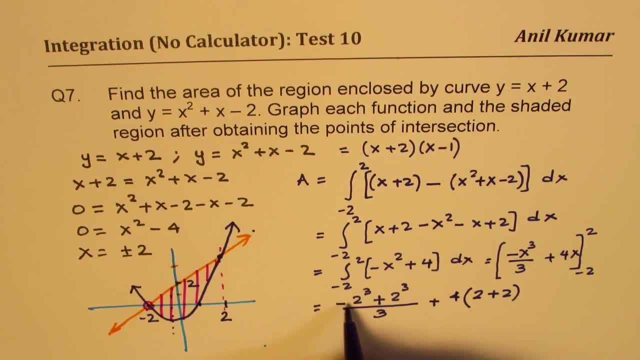 becomes the integral for us. So this minus we'll take outside, actually 2 cube will give us a negative value. Let me write minus like this: right So, which is equal to 8 and 8, 16.. So we get minus 16 over 3 and that is 2 and 2, 4, 4 times 4 as 16, right So? 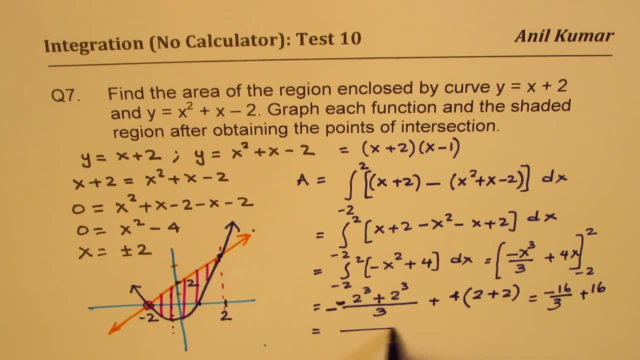 we get this, which is basically equal to 3 common denominator minus 16, plus 3 times 16, which is 48.. And so we get 2 times 16,, 32 over 3 as our answer right. So 32 over 3 unit square we. 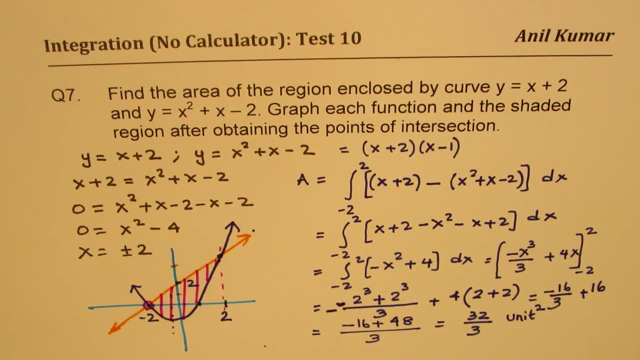 can write clear. So that is how we can actually find the area of the region between these two curves clear. So I hope the solution is okay. Feel free to write your comment, share your views and, if you like, and subscribe to my videos. that's very much appreciated.